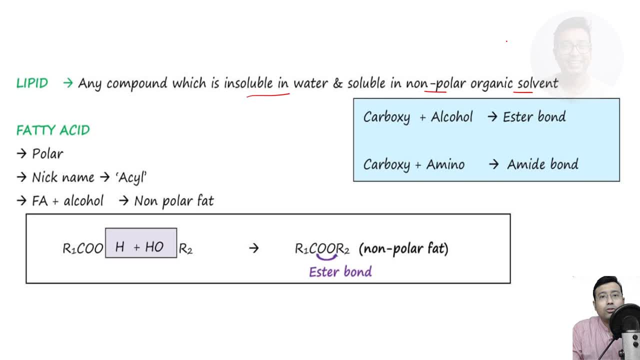 solvent, for example benzene. Okay, so fatty acid, next terms: fatty acids. fatty acids are polar compounds. Their nickname is acyl. So whenever henceforth you hear the name acyl, you should always know it's mentioning, it's referring to a fatty acid. right And fatty acid. 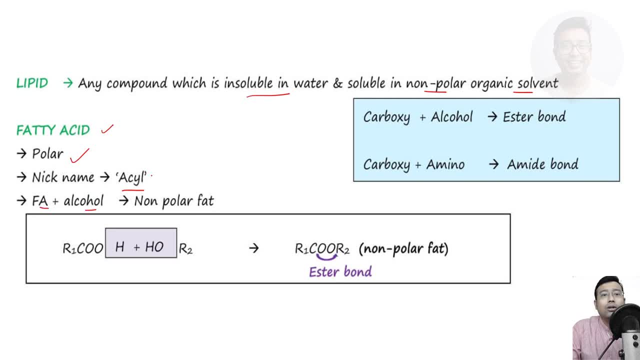 plus alcohol. right, So it's a fatty acid. right, So it's a fatty acid. right, So it's a fatty acid generally leads to non-polar fat, okay, So what do you mean by fatty acid plus alcohol? 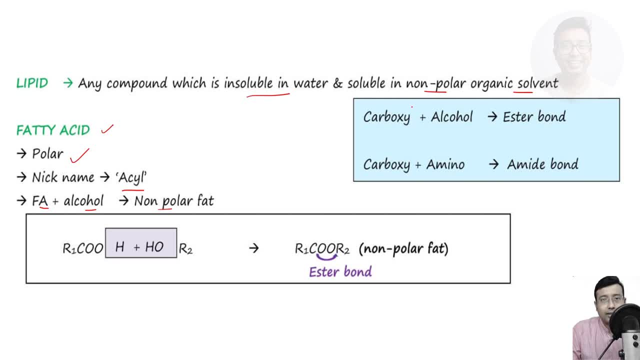 There may be formation of various type of bonds in fatty acid. Remember, fatty acid always ends in a carboxylic group. It's a carboxylic acid, right? So carboxy group plus alcohol makes an ester bond. okay, Carboxy group plus amino makes an amide bond. So here you can see a carboxylic. 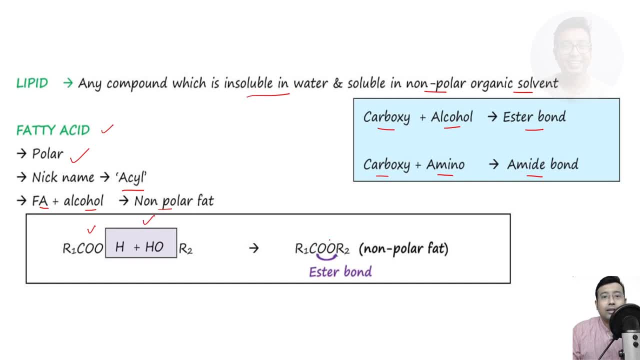 group plus alcohol makes an ester bond right. So here you can see a carboxylic group plus alcohol. okay, This COR2 is actually an ester bond and it's a non-polar fat. That is what we were referring over here. Fatty acid plus alcohol via an ester bond makes it a non-polar fat, okay. So these 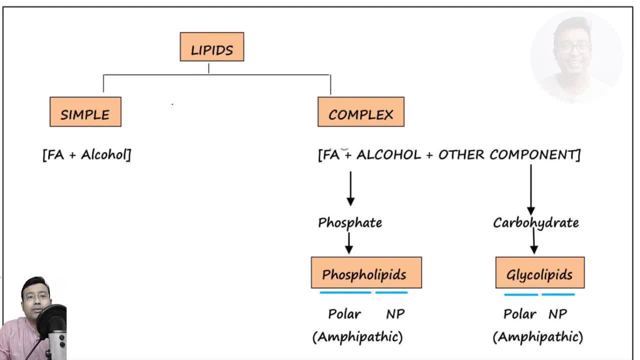 are the basic conceptual areas. Next we classify lipids. Simple lipid means a combination of fatty acid and alcohol. non-polar, we already discussed Complex lipid means those two basic components plus something else. Now this, something else. other component can be phosphate group that. 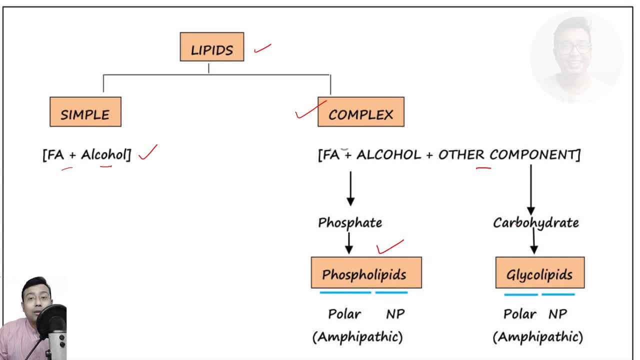 will make phospholipid and it can be carbohydrate that will make glycolipid. Remember, both can be. I mean both of them have got polar as well as nonpolar areas in the structure, So they are referred to as amphipathic lipids, Means some of the areas in the structure are hydrophilic in. 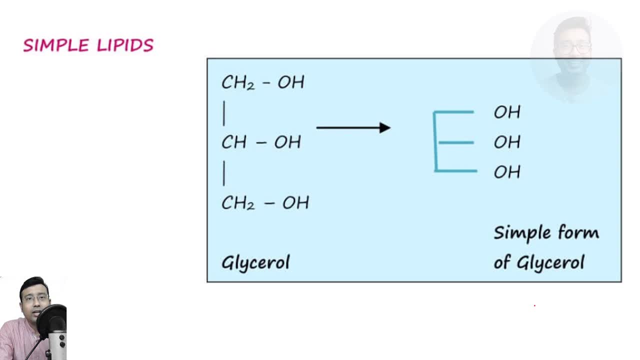 nature and some are hydrophobic in nature. Hydrophilic means water loving and hydrophobic means water hating. Now you can see, here is a structure of simple lipids, glycerol. okay, We can also represent glycerol, like these three OH groups, So this is a tricarboxylic acid. 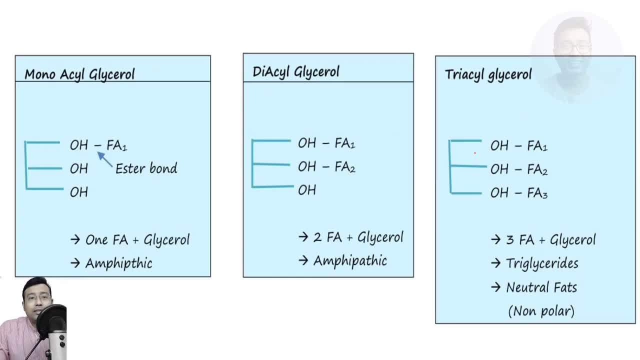 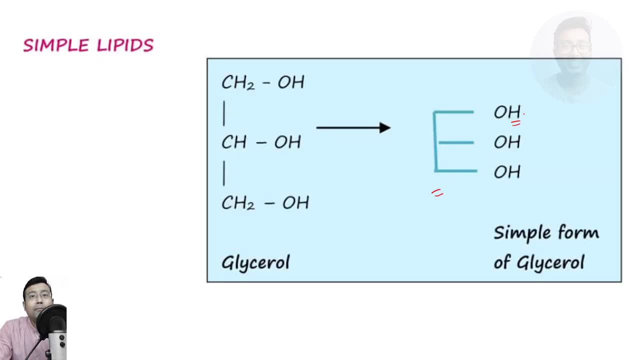 Now those OH groups can be replaced by glycerol, So this is a tricarboxylic acid. So this is a tricarboxylic acid. Now fatty acid. remember this OH group is an alcohol. so whenever a fatty acid is combining with an 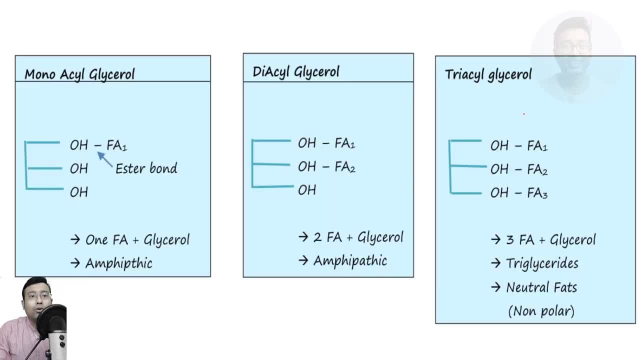 alcohol, it will form an ester bond. so first, when one fatty acid replaces an OH group, it becomes monoacylglycerol. so it means one fatty acid plus glycerol, monoacylglycerol. it is an amphipathic. okay. now, when two fatty acids are forming ester bonds, with both the hydroxyl group. 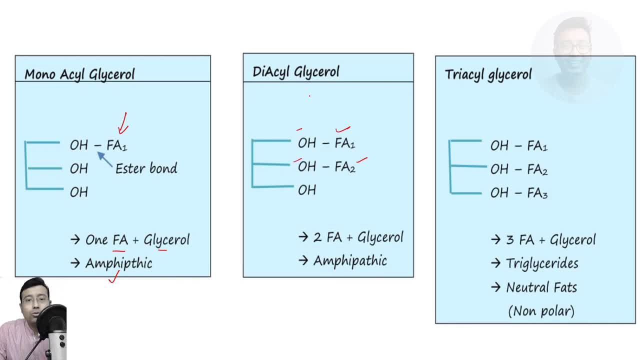 it is diacylglycerol, so two fatty acid and glycerol. it is also amphipathic in nature. however, you see, when three fatty acids are coming and binding with OH groups via ester bond, it is three fatty acid plus glycerol, it is triacylglycerol. it is also known as triglyceride or TG. 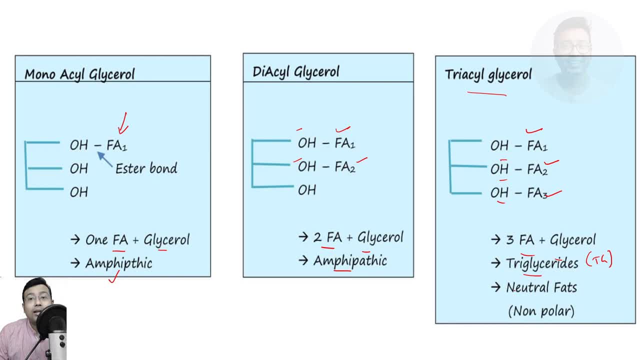 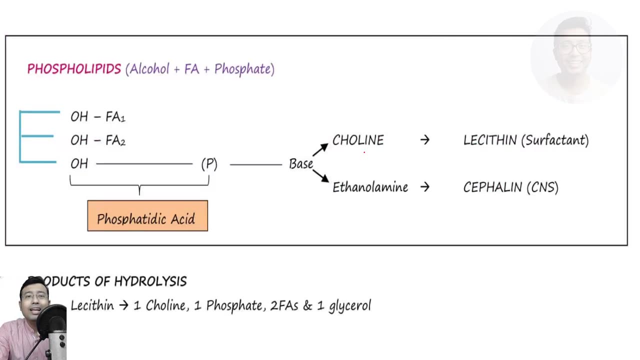 TG okay, and they are neutral. that is non-polar, very, very, very important. so binding of one fatty acid makes it amphipathic, two fatty acid amphipathic, but three fatty acid again makes it non-polar. next we look into phospholipids. you may comment that we are going very fast. okay, yes, we are going. 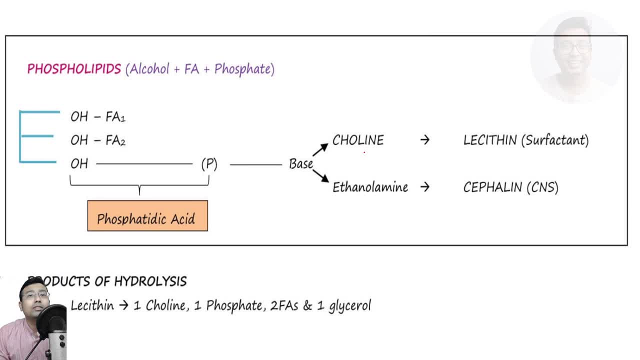 very fast, because these are the bare minimum that you need to know, and these are the most important areas, for mcqa will not be focusing on redundant areas that you don't need, simply okay. so phospholipids means alcohol, fatty acid and phosphate group, right. so fatty acid one and fatty acid two have formed. 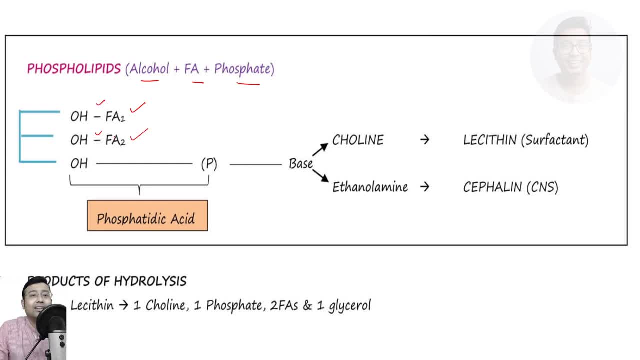 ester group with two OH group of glycerol and in the third OH group this phosphate group is linked- this is known as phosphatidic acid- two acyl group and one phosphate group- okay, this is known as phosphatidic acid or phosphatidic acid- and to the phosphate group. 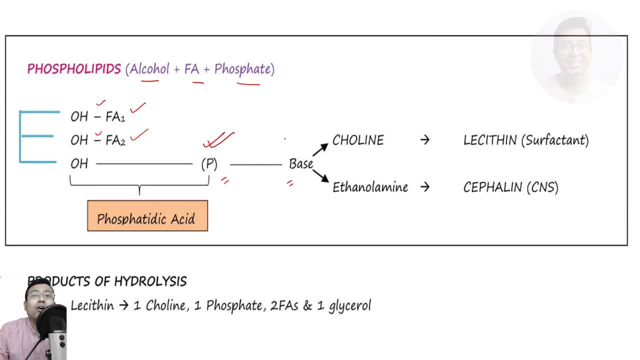 a base may be attached. now, depending on the nature of base, the name will change. if this is choline, it is known as lecithin it is. if it is choline, we also name it phosphatidylcholine. p, h, o, s, p, h, a, t, i d y l- phosphatidylcholine. 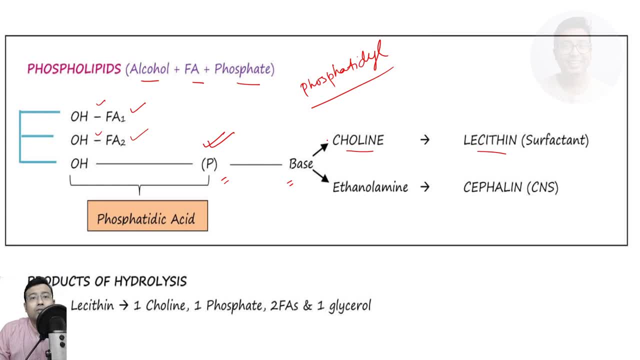 because it is phosphatidic acid and choline. similarly, phosphatidyl ethanolamine is cephaline or kephaline. okay, now, lecithin plays a role as lung surfactant and cephaline plays a role in cns. okay, these are additional questions that may be asked, but we will deal with them later. 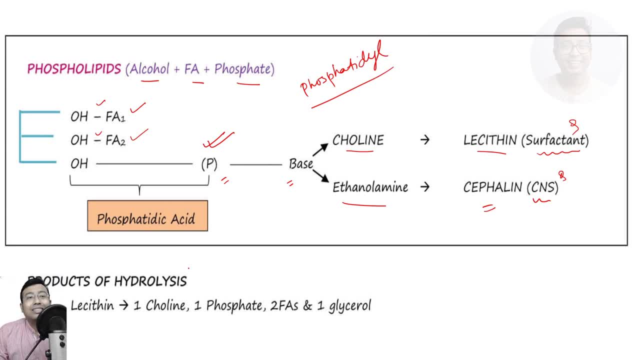 next, we need to know what happens when these type of compounds are hydrolyzed, when they are broken down. so if we break down lecithin, we get one choline, one phosphate, two fatty acid and one glycerol. all right, because these are the ones. 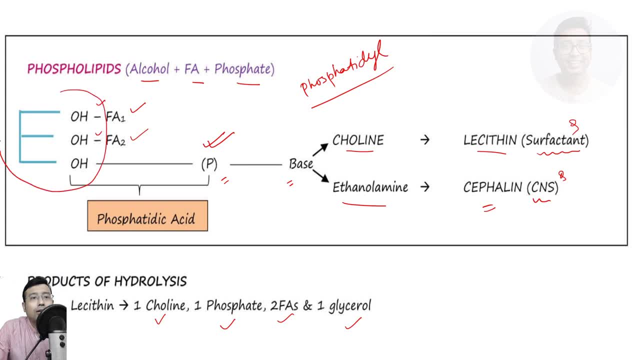 that are attached. the one is glycerol, there are fatty acids and there is a phosphate group- okay, and there is a base. in case of lecithin, the base is choline. so basically, we will get all of them when they are broken down. now, what will break them? these phospholipids are broken down by the enzyme. 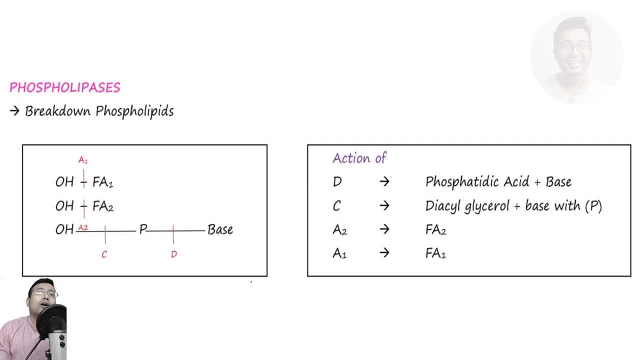 known as phospholipase. okay, now we deal with phospholipase in much more detail. in digestion and absorption of lipid that it may be a part of lipid metabolism, but when you are studying lipid chemistry, we should always know about how a molecule is broken down right? so phospholipases can be of four types. a very gross. 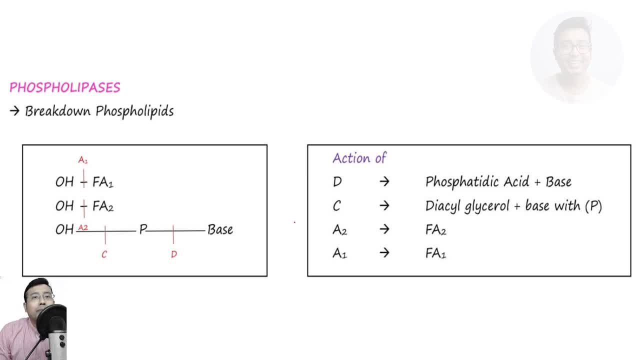 summary: phospholipase a1, phospholipase a2, phospholipase c and phospholipase d- and these are the where those phospholipase actually breaks the molecule. so you see what happens when we use phospholipase a1. so what will phospholipase a1 do? phospholipase a1 will simply break down. 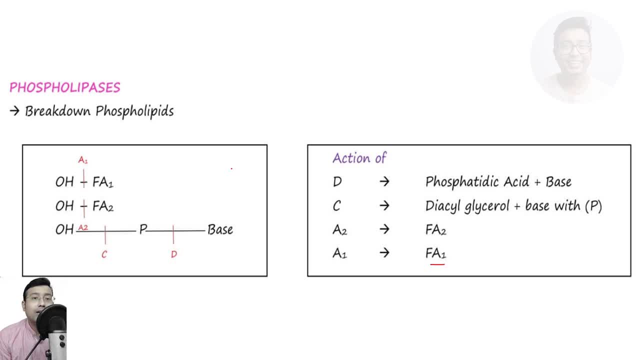 the fatty acid. it will break the first ester bond. similarly, phospholipase a2. what it will do? it will attack this bond. okay, so we will get fatty acid two. okay. next, phospholipase c. what will phospholipase c do? it will attack, over here, the bond between hydroxyl group and the phosphate group. 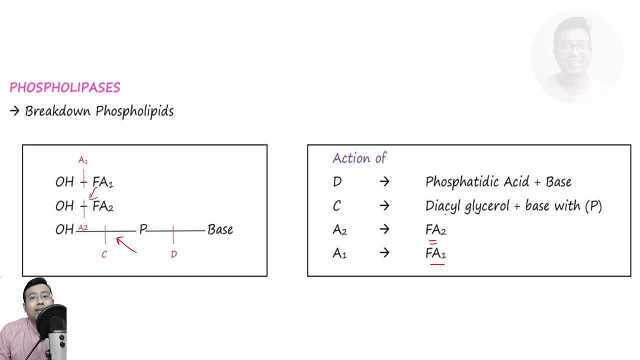 so phospholipase c action will lead to diacylglycerol plus the base with phosphate, so this is the base with phosphate. okay, very important mcq question. and if phospholipase d acts, we get the base and phosphatidic acid. okay, very, very, very important. this slide is one of the 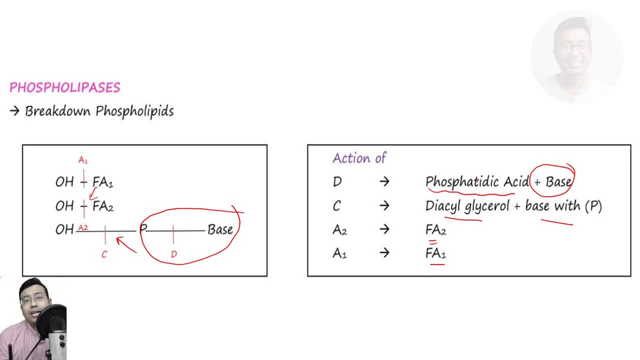 most important slides for mcq purpose, for need, pg preparation, as well as for undergraduate student, but especially for mcq. so please keep in mind and please make your own note about the action of various phospholipase grade of enzymes. remember, since these are breaking down the enzymes, that 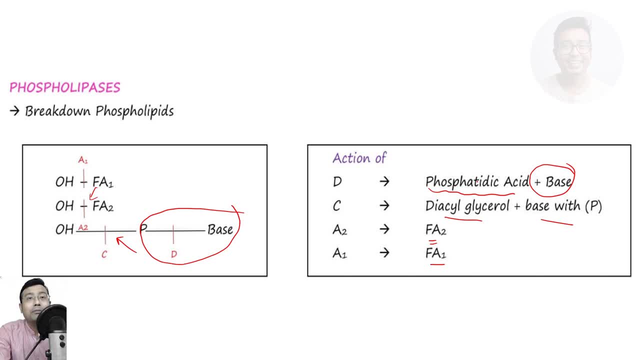 break down can be categorized into two variety. if they break down with the help of water, we call it hydrolase, and if they break down just like that, they are known as lies. so it is your homework to find out what category of enzyme are phospholipases, and then you can write that in the comment section. 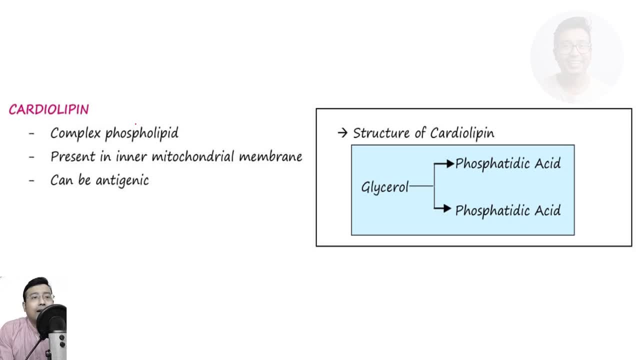 next, a very important phospholipid. that is cardiolipin. you need to know the structure of cardiolipin separately. that is why we are mentioning cardiolipin. okay now, cardiolipin is a complex phospholipid. it is present in the inner mitochondrial membrane and has got many role in 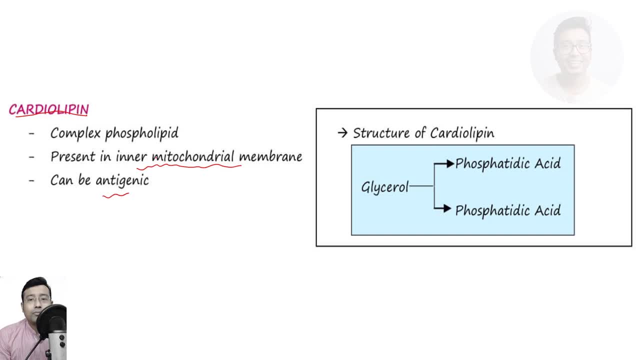 immunity so it can be antigenic, right. so it has got a huge structure. so, basically, what is cardiolipin? it is a molecule of glycerol connected with two phosphatidic acid or two phosphatidic acid that is connecting a molecule of glycerol. you can find the structure. 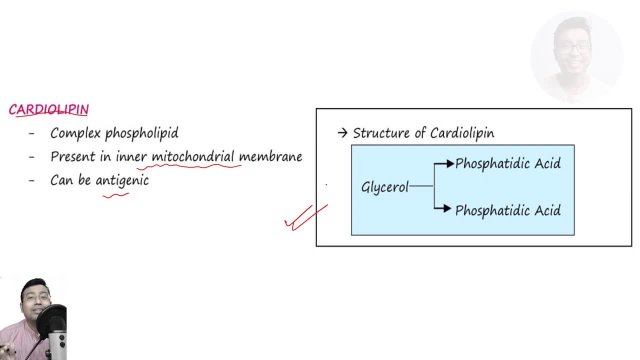 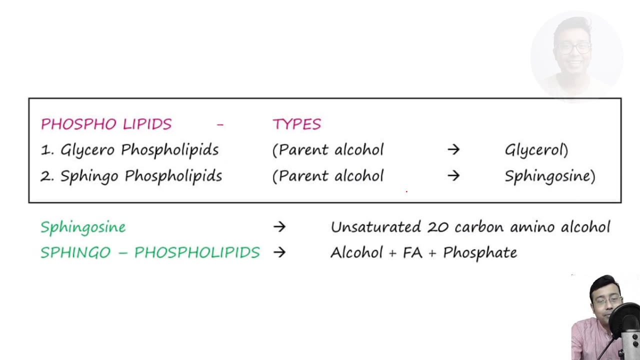 of cardiolipin in your book. it is very huge. but the basic linkage is this: there will be phosphatidic acid on either side and they will be connected via glycerol. next again, there are types. now phospholipids can be classified based on the parent alcohol. okay, if the parent alcohol is. 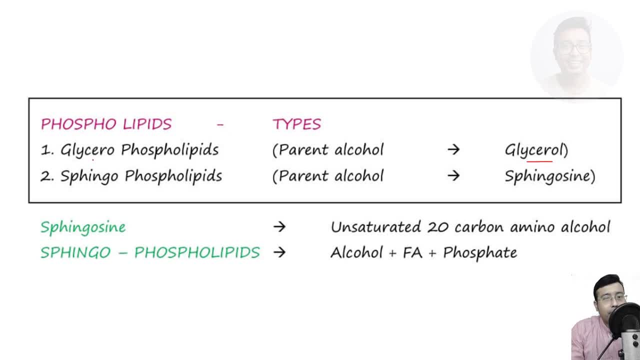 glycerol, they are known as glycerophospholipid, and if the parent alcohol is sphingosine, they are known as sphingophospholipid. okay, now, what is sphingosine? sphingosine is an unsaturated 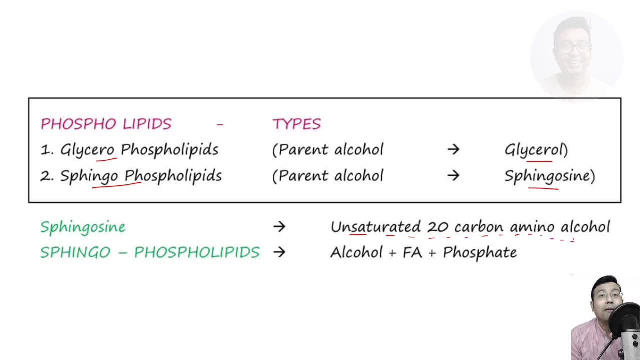 20. carbon amino alcohol. okay, there is an amino group in the alcohol and hence sphingophospholipids: alcohol plus fatty acid plus phosphate group, the alcohol being sphingosine. okay, so i hope these basic concepts are clear. you can take your own time, you can analyze each of this slide and you 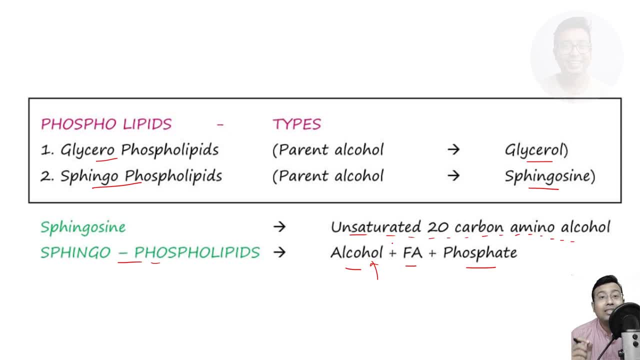 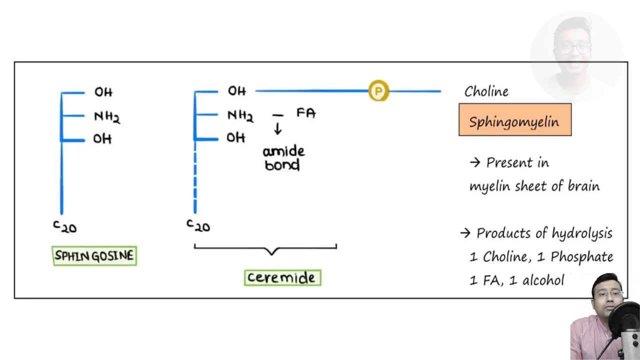 can corroborate with your textbook, but make sure these fundamental concepts are very, very, very clear, right? so you see, uh, this is sphingosine, a 20 carbon amino alcohol. okay, there's an amino group and there are 20 carbons. right, so when this sphingosine combines with a fatty acid, this is known as ceramide. okay, there's a. 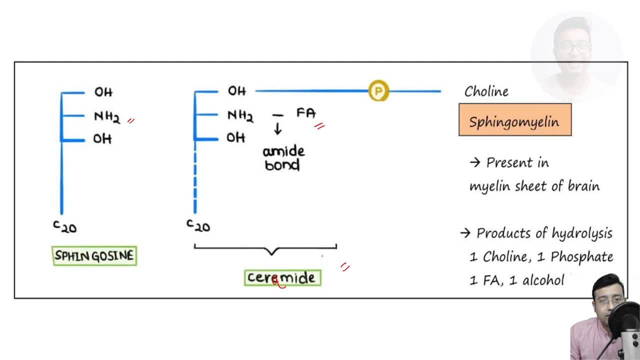 spelling mistake, it will be ceramide. c r, a, m, i d right. so sphingosine plus fatty acid makes ceramide. now if this is connected with a phosphate and a base, for example if this base is choline, it will be sphingomyelin, so b. 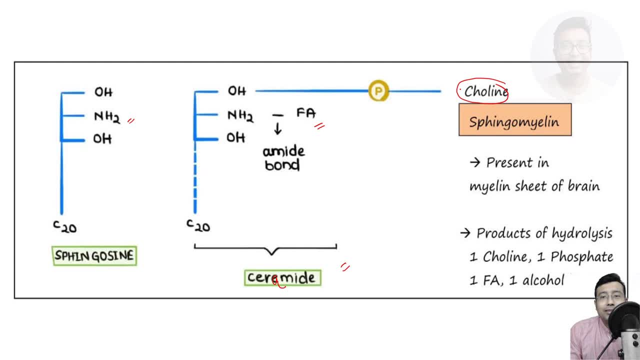 different, i mean based on this base, the differences on this base. this basic structure of ceramide can lead to many such compounds. one of them is sphingomyelin. so let us know one or two things about sphingomyelin. sphingomyelin number one: it is present in myelin sheath of the brain. 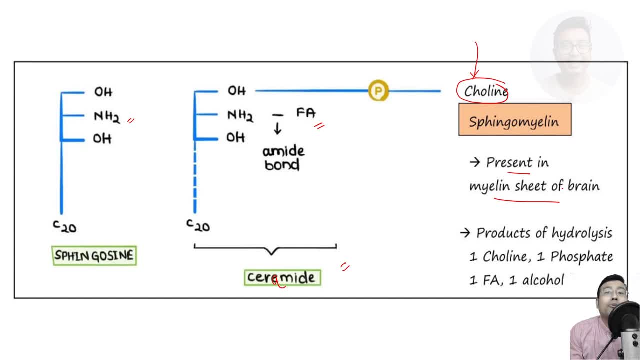 very important. so what will be the product of uh hydrolysis of sphingomyelin? so if myelin is broken down, we get choline, we get one Venous seed. so two other compounds, so daaramo, frankplauhافingomyelin. number one. it is present in myelin sheath of the brain. very important. so the last one: uh, cornelian, we get choline, we get heterdulosis and we therefore see the birth of Sphingomyelin, first type of 95 DONGH. niemand knows how this is made, pretty much almost a straight line, because architect is a heavy care outrosideoh. 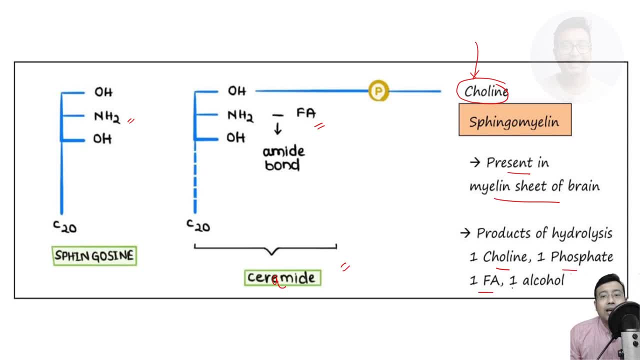 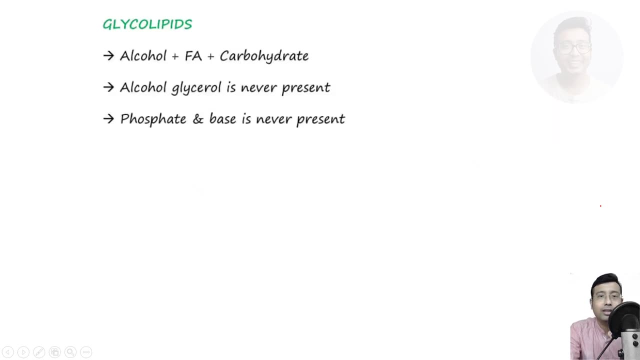 phosphate. we get one fatty acid and we get one alcohol, this alcohol being sphingosine. Now, I hope you are getting a clue. We have told hydrolysis, So it means breaking down with the help of water, right, Anyway, now we move to glycolipid. okay, We need to know a brief. 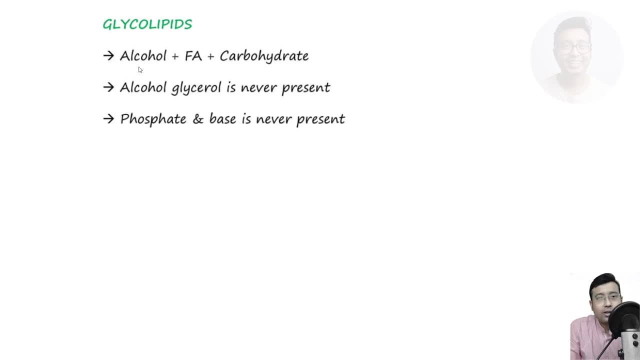 about glycolipid. Glycolipid consists of alcohol, fatty acid and carbohydrate. okay, Remember this. alcohol is not glycerol. It is never present in glycolipid, So students often confuse glycerophospholipid with glycolipid. In case of glycerophospholipid, the parent alcohol is 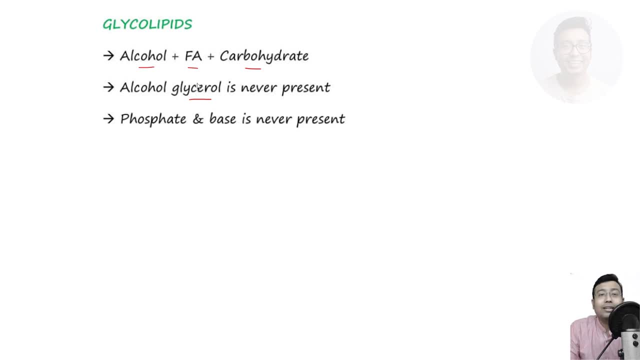 glycerol, But we are discussing glycolipid over there. Glycerol is never present. Similarly, phosphate and base is also never present. So these are actually part of MCQ questions that are given in all except form, So they will give. 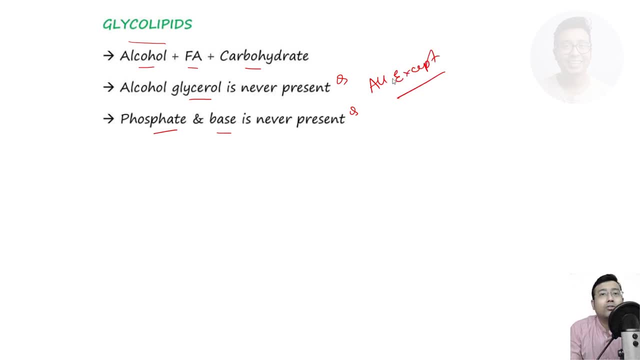 you name of four or five alcohols and you need to select which one of them is not present. Then, of course, you need to mark glycerol, And all of them are present in glycolipid except. So if phosphate and base is our option, they are also not present in glycolipid. So what's the 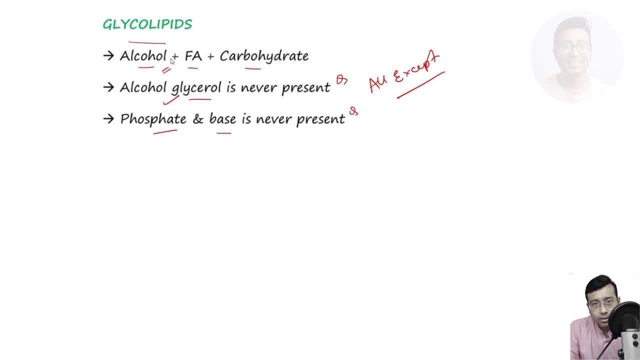 alcohol that is present in glycolipid. The alcohol is actually sphingosine. okay, And based on this difference in carbohydrate, this glycolipid is not present in glycolipid. So we need to know. glycolipid can be classified into two different types. Basically they are ceramides, So if 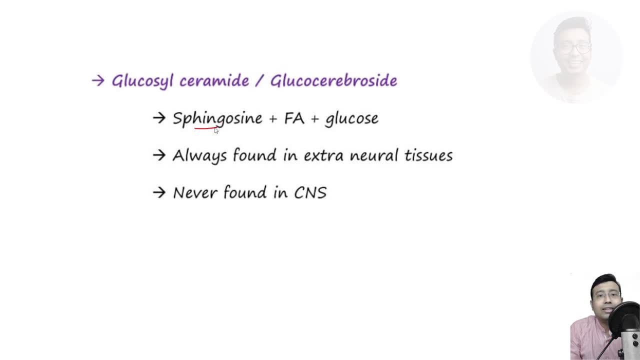 the glycolipid has got sphingosine and fatty acid and glucose. it is known as glucosilceramide or glucocerebroside. What is the function? They are found in extra neural tissues and never found in central nervous system. Very important, okay. And the next type, that is galactosilceramide. 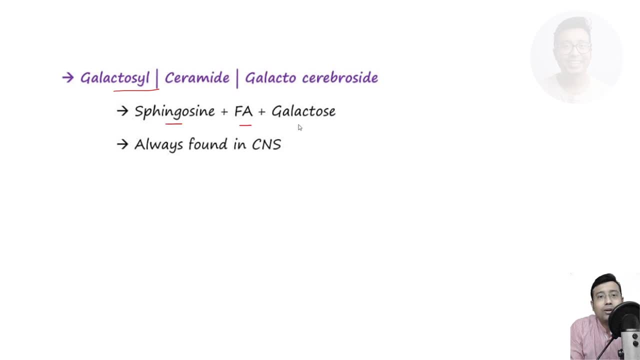 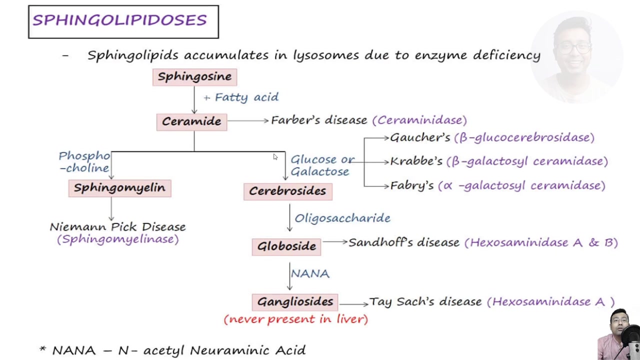 it is sphingosine. So these are two varieties of glycolipids. Next we go on to sphingolipidosis means sphingolipids and the diseases. okay, This chart is basically very exhaustive And, as a first year student, 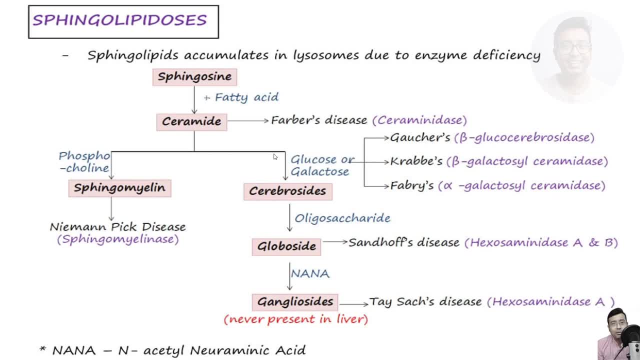 I agree it's a bit- not a bit- difficult to remember all of these, But if you are going for neat PG, trust me, these are hot areas And questions will be set from these areas mainly So you need to remember what is the name. 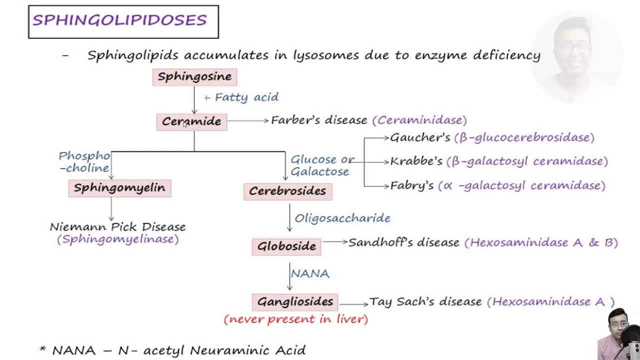 of the disease and what is the enzyme that is deficient? okay, So let's look at the whole flow chart and analyze them. So sphingosine plus fatty acid forms ceramide Here. if this enzyme is deficient, that is known as ceramide. So if this enzyme is deficient, that is known as ceramide. 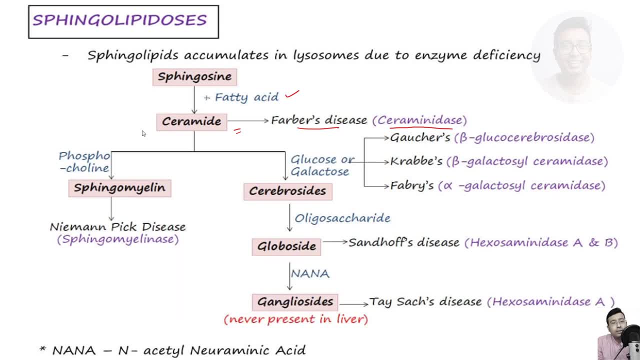 You can see here, ceramides have many aways. it leads to Farber's disease From this ceramide it can have two fates. If a phosphocholine is attached, that is a base and a phosphate group, we get sphingomyelin. In that context you need to remember name of this disease known as 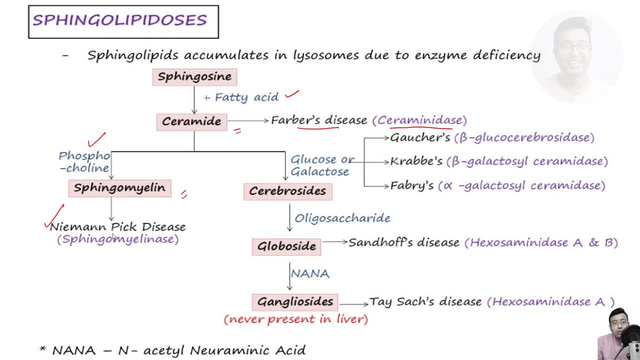 Nieman-Pig disease. It's due to deficiency of an enzyme known as sphingomyelinase. okay, And another fate is: either carbohydrates will be attached right. So the carbohydrates can be either of these cofactors which are present in the body or they are at the start. So if you have, a cofactors that are related to polyunsaturated intrigued in the body, they are not able to have the concerns of their bodies. so they don't actually have the concerns of their bodies If you have a to Alfaloid and a cofactors. 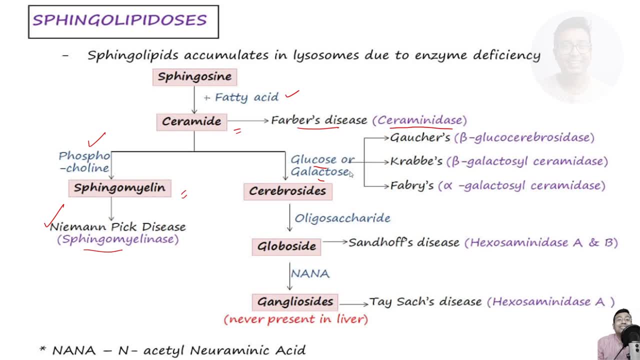 glucose or galactose From this area. there may be three different diseases. Number one, Gaucher's disease, Very important. This is due to deficiency of beta-glucocerebrosidase- Okay. Next, Crabbe's disease Due to deficiency in beta-galactosilceramides. And again Fabry's. 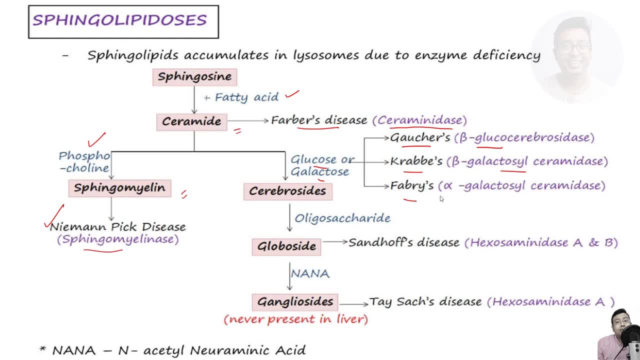 disease. It is due to deficiency of alpha-galactosilceramides. Okay, So all three are important: Gaucher's, Crabbe's, Fabry's, Right, Next from cerebroside, when an oligosaccharide. 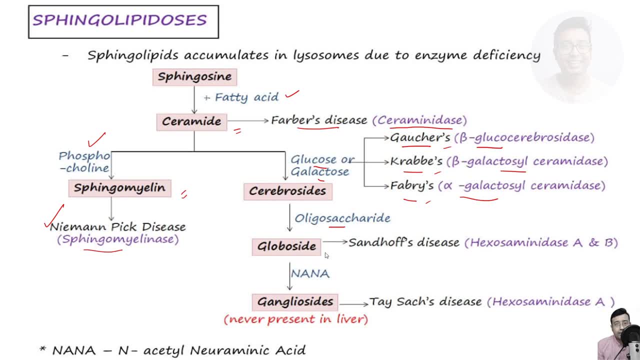 molecule is added to the residue, we get globoside Right. And, in this context, important disease is Shandoff's disease. It is due to deficiency of hexosaminidase A and hexosaminidase A And, in this context, important disease is Shandoff's disease. It is due to deficiency of 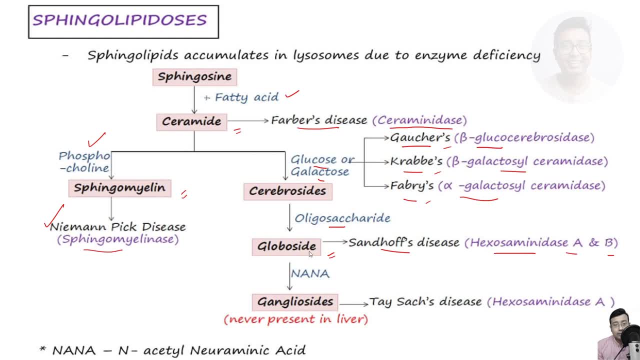 beta-galactosilceramides- Okay. And lastly, if we add a residue of non-acetylneuraminic acid, that is Nana, If we add one Nana to globoside, we get ganglioside Right. And this has got also. 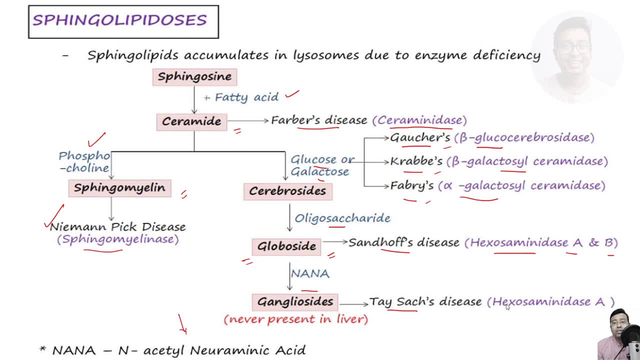 another disease in relation to this, That is, hexosaminidase, A deficiency That is Tayshack's disease. Remember, hexosaminidase, A enzyme, can catalyze formation of both global side and ganglioside. So in case of Tayshack's disease, this enzyme is deficient, but there is. 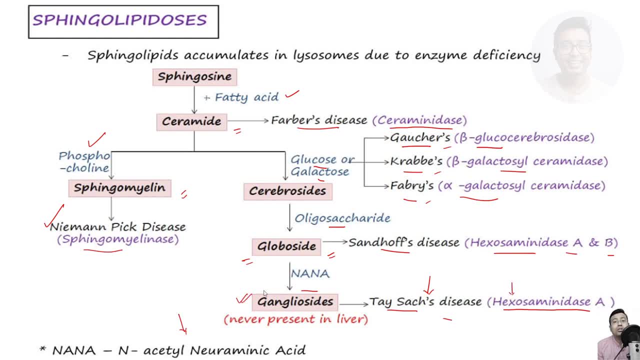 deficiency in gangliosides, This problem: there is accumulation of ganglioside, But this disease- one thing you need to know for MCQ purpose- this ganglioside dosis never happens in liver. This is a disease of central nervous system. Okay, Others are affect liver- Very, very, very important. So 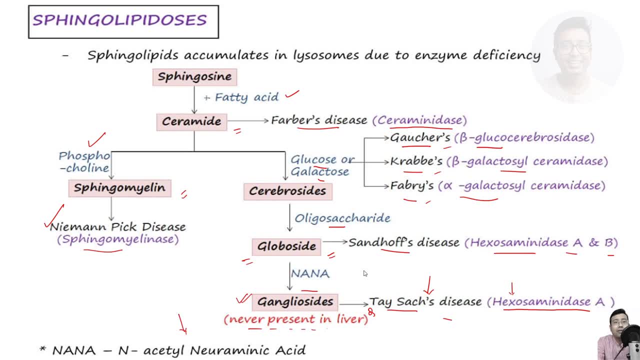 all of them have got hepatomegaly, that is, liver enlargement, except ganglioside dosis, that is Tayshack's disease. Okay, We will be discussing the salient features and all except what specifically you need to remember in upcoming slides. 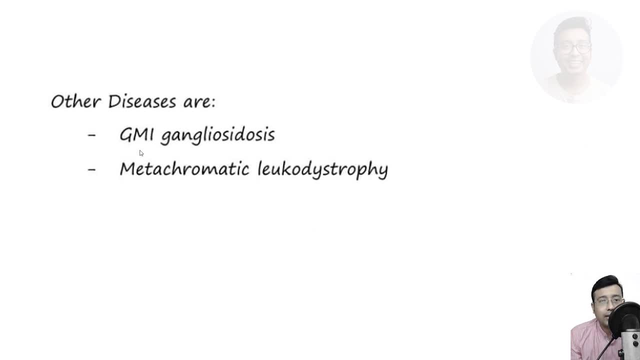 Other diseases that you need to know is GM1, ganglioside dosis and metachromatic leukodystrophy. It is due to deficiency in aryl sulfatease A. Okay, Aryl sulfatease A. Believe me, there is an. 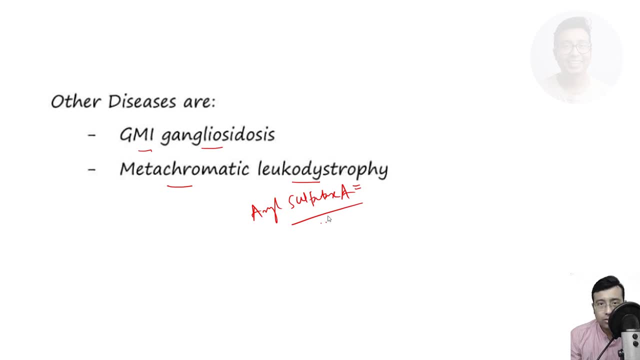 exhaustive chart in your chart. So if you have an exhaustive chart in your chart, you need to read the textbook. As a first year student, or even as a postgraduate student, you only need to know the name of the diseases and the enzymes that are deficient Only if you are appearing for highly 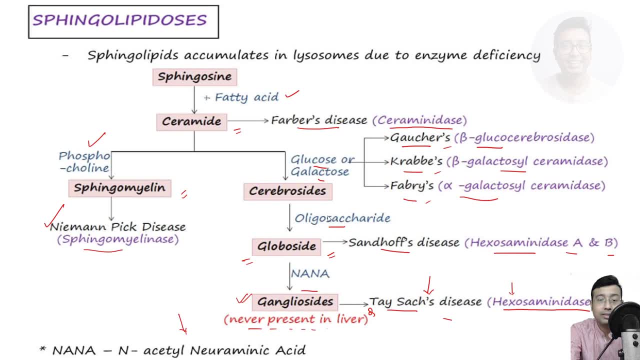 competitive exam. then you may get image-based questions. In that type of question. the areas in these steps will be grayed out and then you need to identify where which enzyme are playing a role. So that is an extremely difficult question. I am not betting on that, But as a 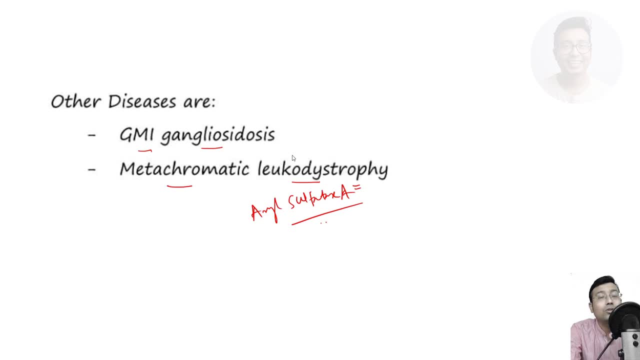 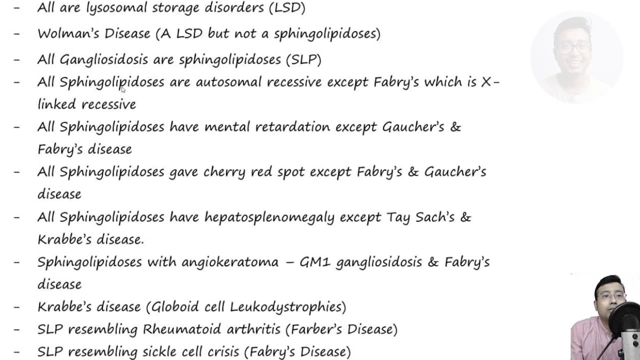 beginner, you need to know the name of the diseases and the enzymes that are deficient. As a beginner, or as a regular reader, you should at least know the name of the diseases and their deficiency disorders. So here is a comprehensive chart. So all of these, so all sphingolipidosis. 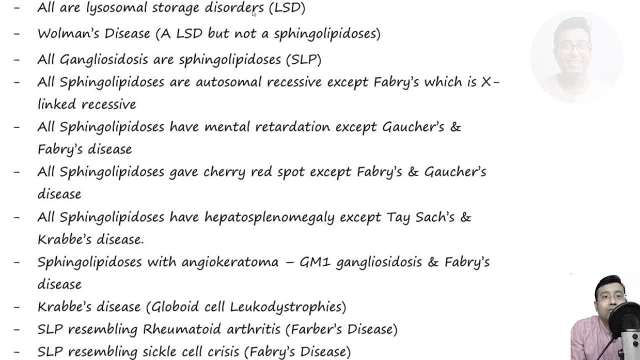 I mean sphingolipids, and their diseases are LSD, that is, lysosomal storage disorder. Okay, Except Wollman's disease is a lysosomal storage disorder but not a sphingolipidosis. It is not a sphingolipidosis. We will be discussing Wollman's disease separately. Okay, 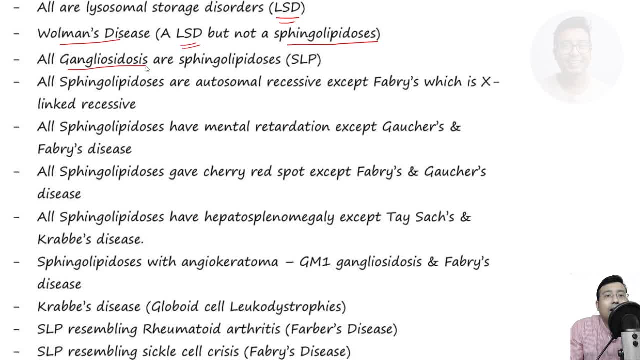 Next, all gangliosidosis are sphingolipidosis. Okay, It means sphingolipids get accumulated. Okay. Next all sphingolipidosis are autosomal, recessive in nature, except Fabry's disease. 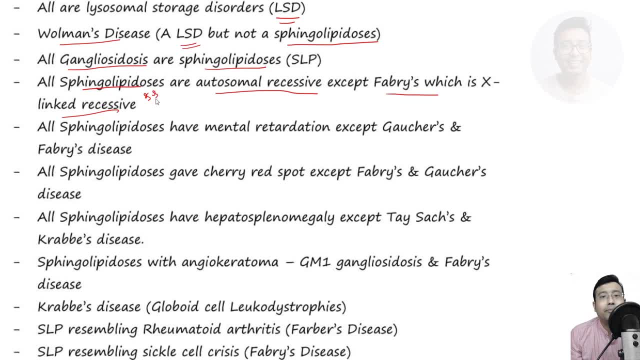 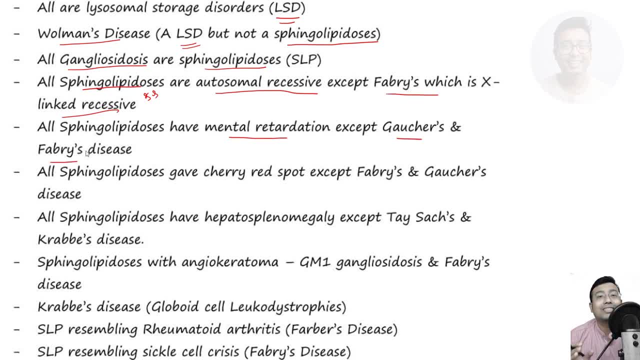 recessive. All of them AR that is autosomal recessive. All of them are AR that is autosomal recessive. All of them do not mean that they are AI. They mean that they are not AI. They are just some Blitzemachyploid. so it doesn't matter at all whether it is AI or someone else's Sil trivial, Okay good, I think there is an entire class today which I will cover, and I think there is an entire class today which I will cover in AR, and look at this with a hundred percent of focus. 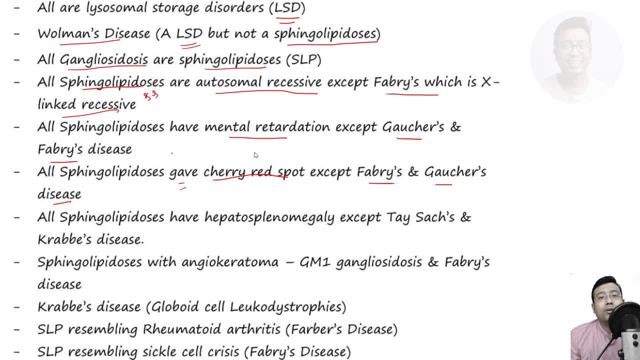 But as a first year student you should know that cherry red spot is absent in febris and gauchers. okay. Next, all sphingolipidosis have hepatosplenomegaly. It means enlargement of liver and spleen, except teshack and crabs. okay. 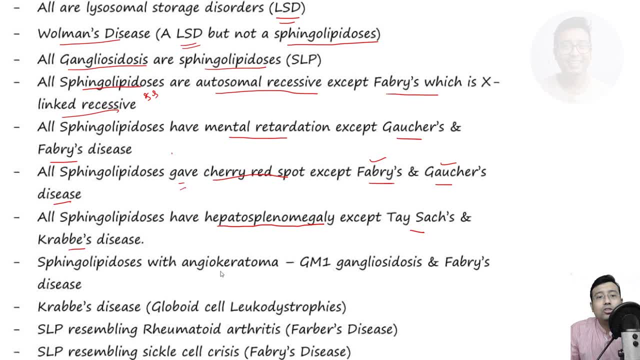 Next, sphingolipidosis with angiokeratoma means there are lesions in the skin. okay. Blood vessels- Blood vessels on the skin get enlarged. So these are GM1, gangliosidosis and febris disease. okay. 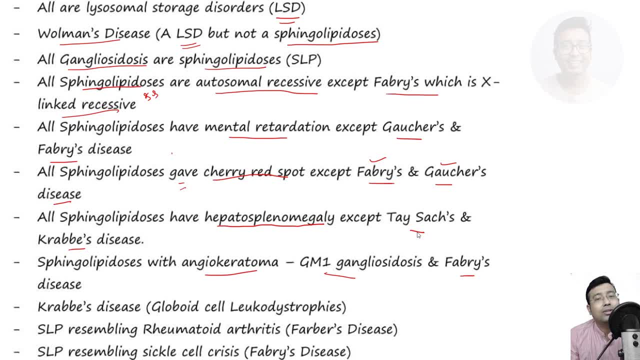 I agree, the list is exhaustive. If you can remember, fine. If you cannot remember, you should at least revise them the day before exam Next. crabs disease is also known as globoid cell leukodystrophy. okay, A sphingolipidosis that is resembling rheumatoid arthritis is Farber's disease. 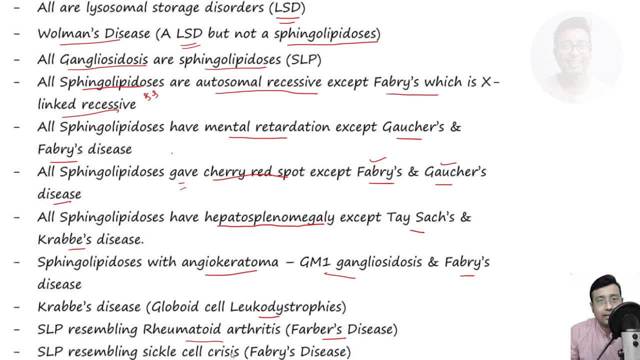 And a sphingolipidosis resembling sickle cell crabs. Sickle cell anemia- we will be reading later- is Farber's disease. Yes, this is an exhaustive list. There is no other way to remember. Only way to remember is reading it over and over again, discussing with your friends. 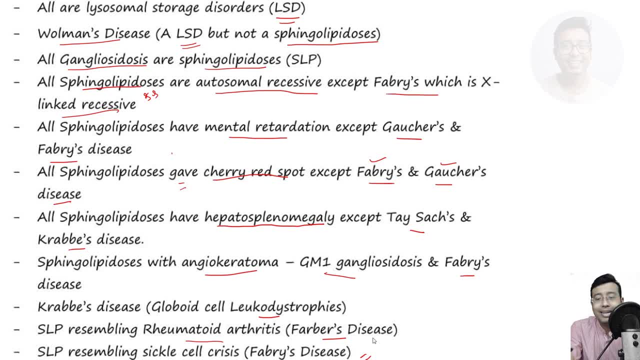 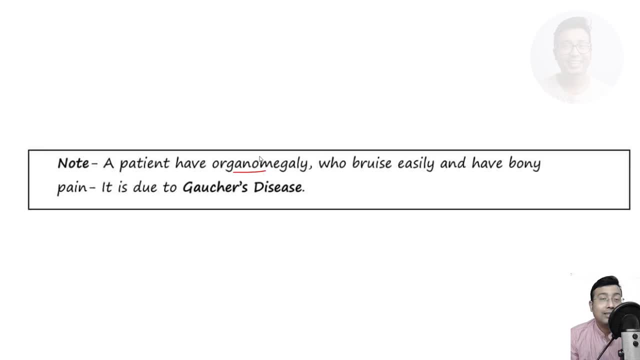 writing it down. Anyhow, you need to remember, but you need to remember. okay, Note a patient of organomegaly. okay, This will come as a long case as a part of your early clinical exposure, or it may be a. 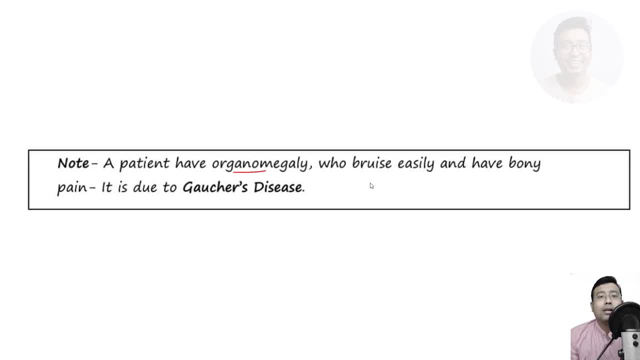 short case in your viva, especially in medicine exam. So having organomegaly who bruise easily and have bone pain. the diagnosis is Gautier's disease. We'll be discussing Gautier's disease. we'll be making a separate video on Gautier's. 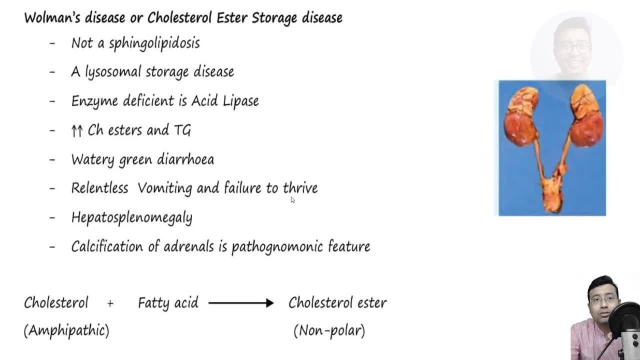 disease in upcoming lessons Next. so the one we discussed that is an exception of sphingolipidosis is Vollman's disease. So let us discuss a few words about Vollman's disease. It is not a sphingolipidosis, but it is a LSD, that is, lysosomal storage disorder. 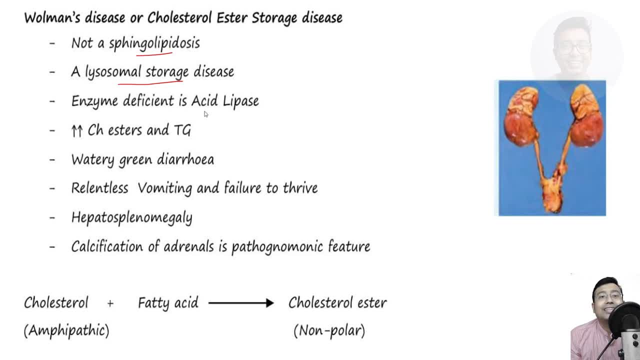 So what is deficient? The enzyme? The enzyme that is deficient is acid lipase. What happens? Increased concentration of cholesterol, ester and triglycerides in the serum. So it is a disorder of lipid metabolism. okay, What is the symptom? 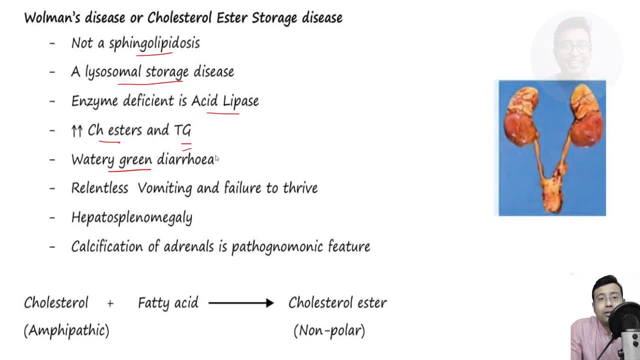 Watery green diarrhea- very important, okay, It is a disorder of childhood actually. So what happens? Relentless vomiting and failure to thrive. okay, These are the two features. Hepatosplenomegaly, That is, enlargement of liver and spleen. 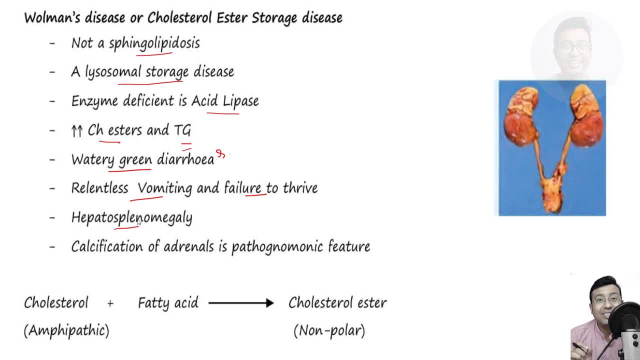 And the pathognomonic feature means the one which helps in diagnosis, is actually calcification of adrenal gland very important. So you see kidney. on the renal there is suprarrenal. Suprarrenal also means adrenal, that is above kidney. 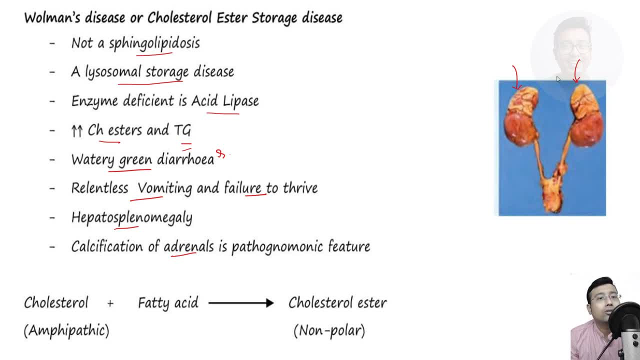 So suprarrenal glands get calcified. This is the diagnostic feature of Vollman's disease. So you see, in addition, since you saw cholesterol- cholesterol is also mentioned in your competency Number one- you need to know the structure of cholesterol. 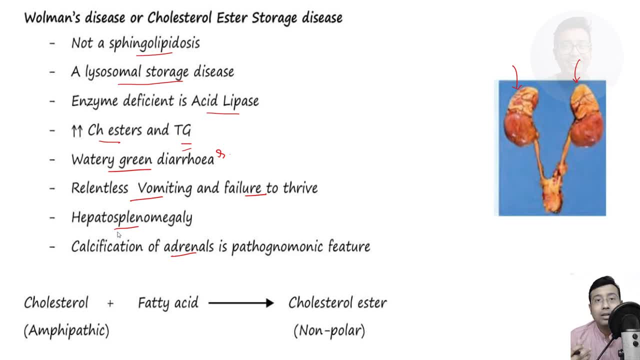 the cyclopentanoparhydrofenanthrin, that is CPP ring. Also, you need to know, cholesterol is itself an amphipathic molecule, okay, But when it combines with fatty acid it becomes nonpolar. Combining with fatty acid, cholesterol becomes cholesterol ester. 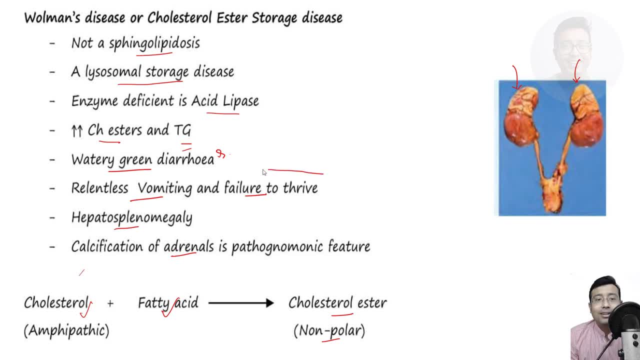 Being a first year student, it may be difficult to come across all these terminologies, right, But just know this. failure to thrive: Thrive means inability to maintain growth or poor growth, okay. Inability to sustain or catch up with growth of other peers: okay. 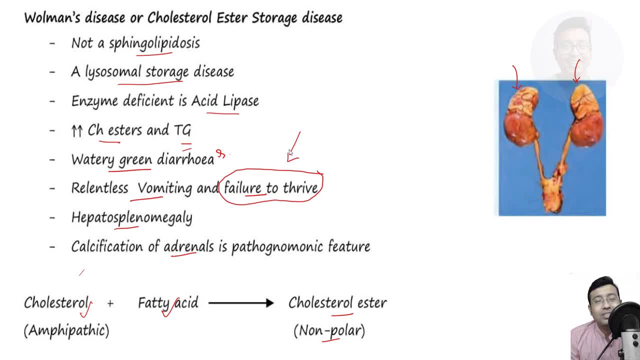 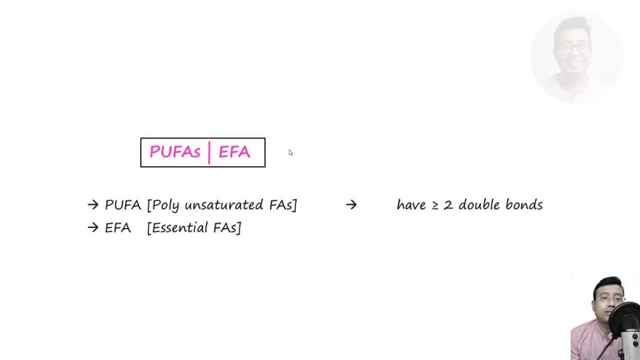 So a child with failure to thrive means you will have stunted growth compared to others Other child of same age group, age and sex. So next move to our last section of discussion, that is, polyunsaturated fatty acids and essential fatty acid. 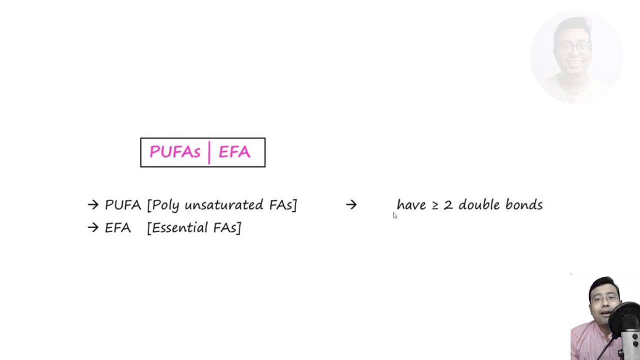 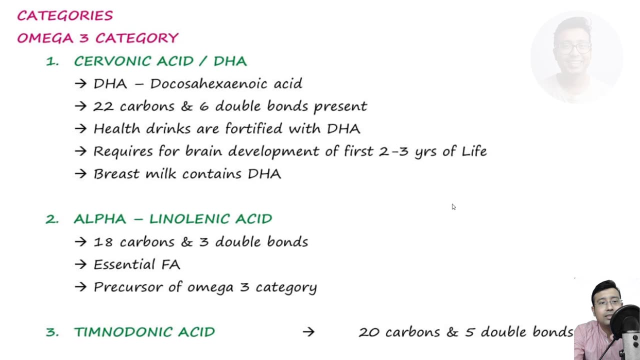 The most common characteristic is they have to have more than two double bonds. okay, So they are of two categories. Number one is omega-3 and number two is omega-6.. There can be many, much more, But those are very important from exam point of view. 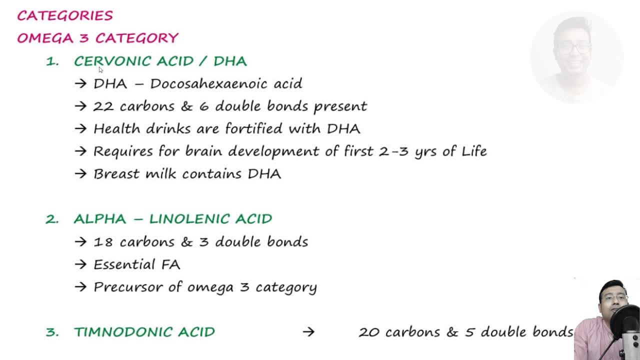 So let's first discuss omega-3.. So sarvonic acid, or docosahexaenoic acid, it is one of the most important omega-3 fatty acid. So docosahexaenoic acid, it is 22 carbons and 6 double bonds. 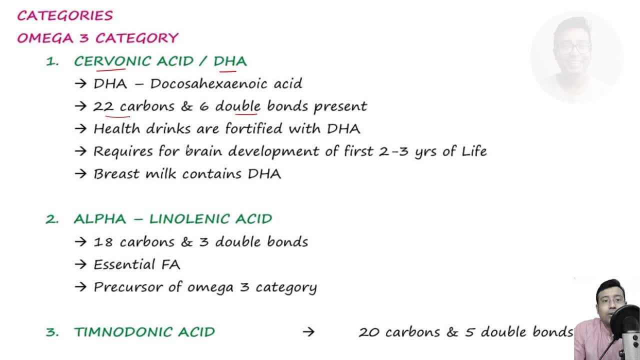 It is actually present in many health drinks. okay, So health drinks, Health drinks, are fortified with DHA And it is also required for brain development in first two to three years of life. And remember, breast milk contains docosahexaenoic acid or DHA. okay, 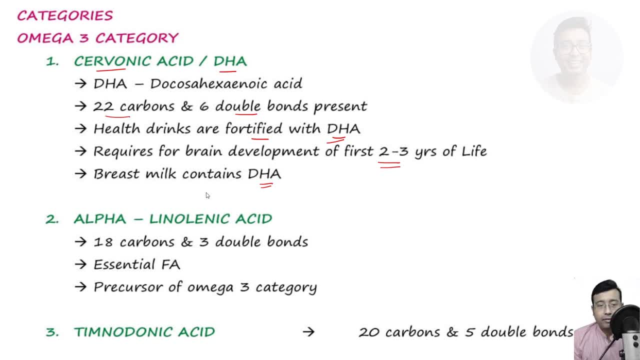 Next most important omega-3 category of fatty acid is linoleic acid. okay, It contains 18 carbons and 3 double bonds. It is an essential fatty acid and it is a precursor of omega-3. So linoleic- from linoleic acid- other omega-3 fatty acid- can be synthesized. 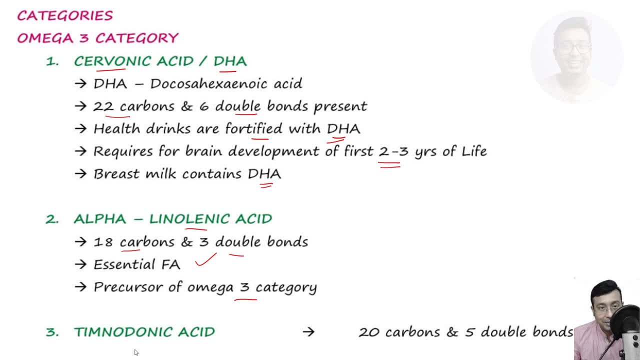 Next, but most important- not most important, actually, nice to know- is temodonic acid. It contains 20 carbons and 5 double bonds. Not very essential, but if you are appearing for gold medal or class assistant exam, it may be asked, okay. 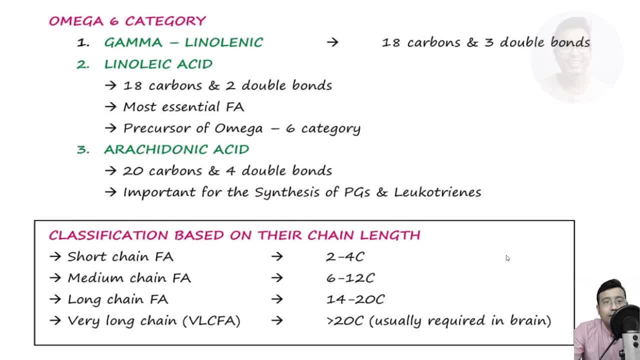 So, lastly, this is omega-6 category, So omega-6, number one is gamma-linolenic, Gamma-linolenic acid. very important. okay, The how omega nomenclature happens. you can go through your textbook, okay. 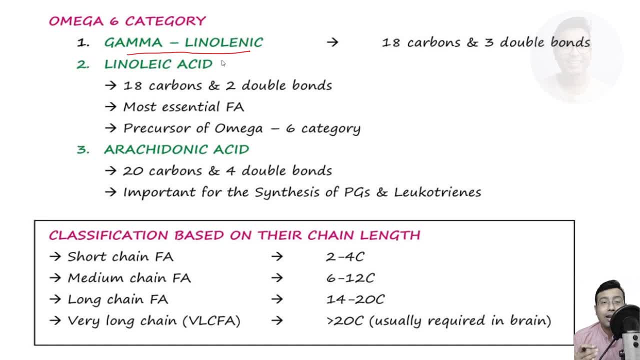 It is the number of the position of double bond from the last, not from the carboxyl end from the other end. okay, So gamma-linolenic acid consists of 18 carbons and 3 double bonds. Next is linoleic acid. 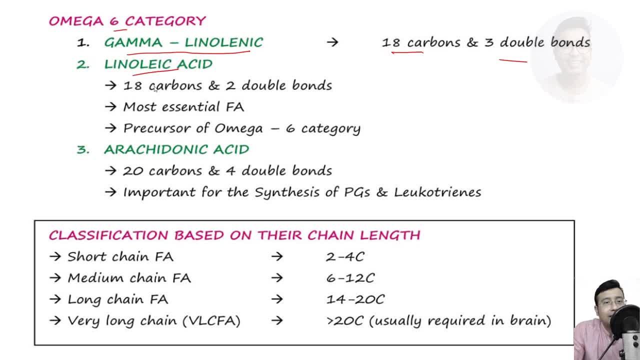 Linoleic acid is an omega-6 category. It has got 18 carbons and 2 double bonds. It is the most essential fatty And it is the precursor of all omega-6 category. okay, Remember, lenic is omega-3, except gamma-linolenic, that is again omega-6, and linoleic is omega-6.. 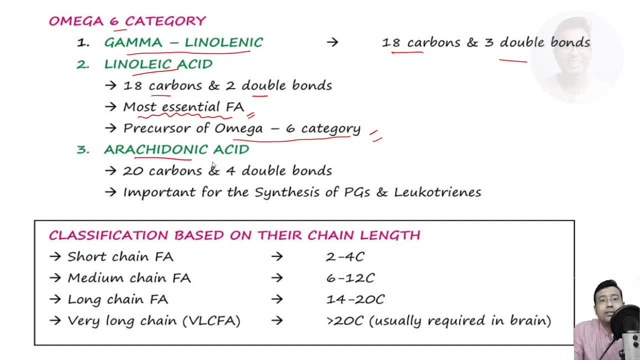 And lastly arachidonic acid. Arachidonic acid: it has got 20 carbon atoms and 4 double bonds. It is the precursor of synthesis of prostaglandins and leukotrienes. Prostaglandins and leukotrienes will be taught in detail in physiology and it is also part of lipid chemistry. 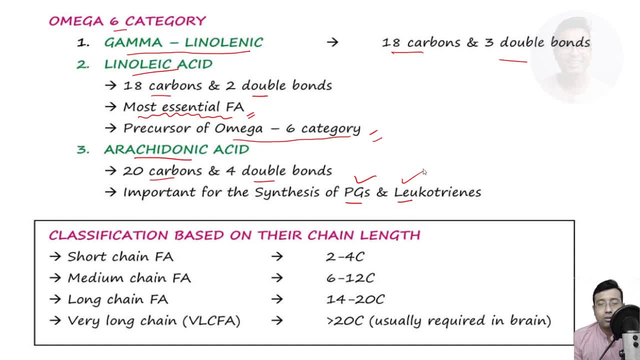 The enzymes cyclooxygenase, lipoxygenase, all those have got medical importance, But as a part of lipid chemistry, you should know at least arachidonic acid is the precursor of prostaglandins and leukotrienes. 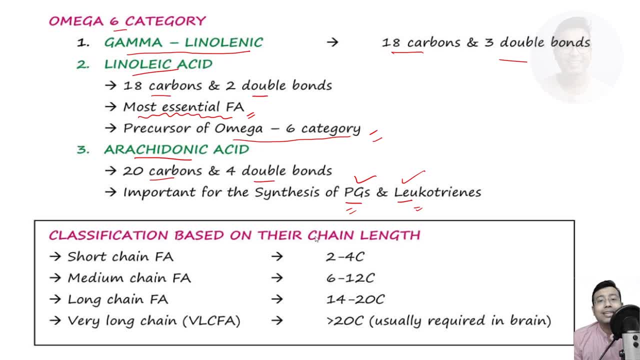 So how can we classify amino acid based on their chain length? Very important Short chain. did I say amino acid? I was wrong. I mean fatty acid. So short chain fatty acid are actually 2 to 4 carbon. Medium chain 6 to 12..